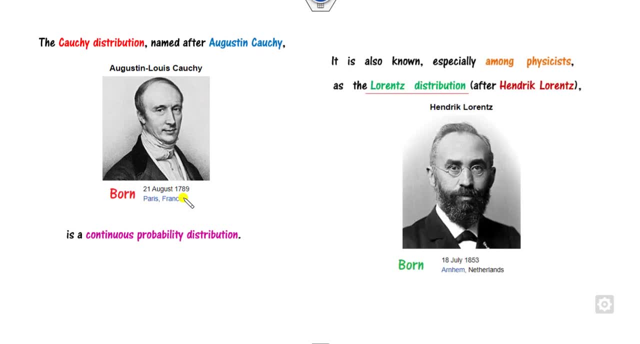 distribution function. In most of the cases, this Cauchy distribution is also called as the Lorentz distribution. because of this famous person called as the M Hankings, It is also called as a Cauchy-Lorentz distribution or the Lorentz function, So it is widely popular in the. 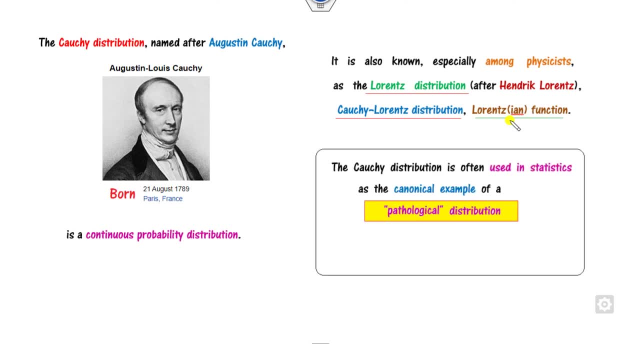 physics sites are there. This Cauchy distribution is the canonical example of the pathological distribution of the Cauchy distribution, So it is widely popular in the physical distribution. What is the meaning of the pathological distribution? The function whose mean and variances are undefined. So this Cauchy distribution has no mean and its no variances are. 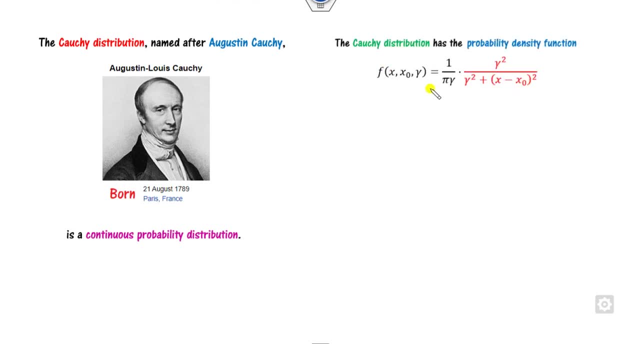 there. This is the probability density function of the Cauchy distribution. There are the two unknown parameter called as the x0, and second one is a gamma, where x0 is defined as the location parameter or called as the shape parameter, defined as the peak of the distribution, and the gamma is. 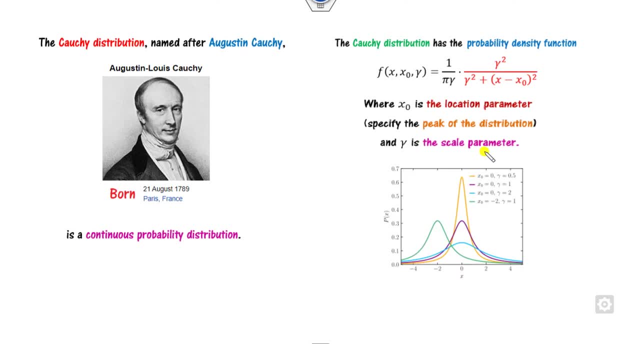 called as the scale parameter. If you draw the probability density function of this Cauchy distribution, then we will see, like here, Clearly say, that this yellow color will say: location is my 0 and this scale parameter is a smallest one, that is a 0.5, and the peak will be high. Similarly for this green color and this: 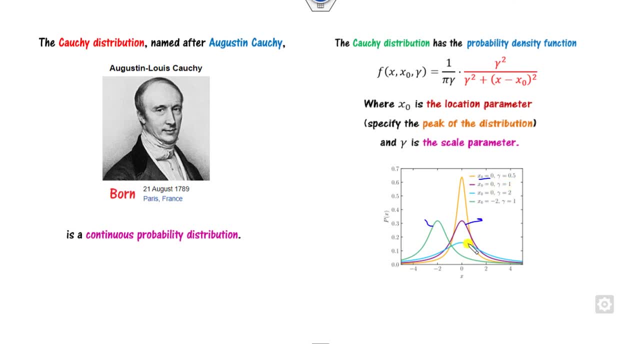 blue color will shows that gamma is my 1 and 2 and similarly, for this blue color you can see there is a wider width as compared to the other one. So that define the parameter effect of the scale as well as the location. So this is the probability density function of this Cauchy distribution. 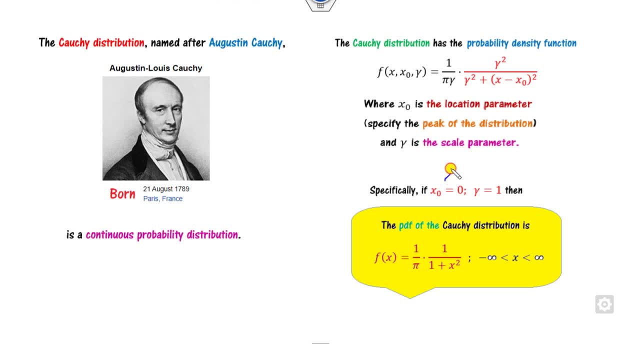 If we set the particular parameter as the location, as a gamma, as a 1 and the location x0 as a 0 in this distribution, then we will see the PDF of this Cauchy distribution as here. Now. our target is to find the characteristics function of this Cauchy distribution. What is the characteristics? 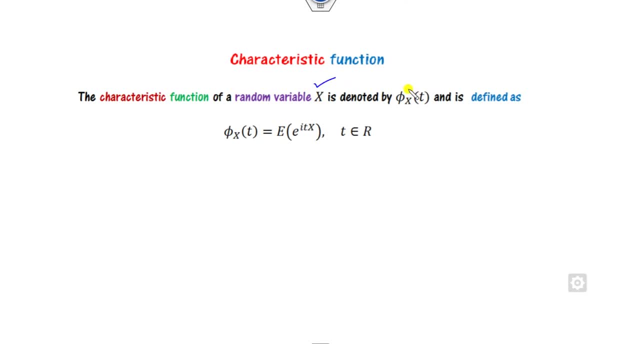 function is Characteristics function of any random variable. x is denoted as a phi, which is defined as expected value of the e raised to power, iota, t, x. So if we have a discrete random variable, then we can write this expected value as a summation. 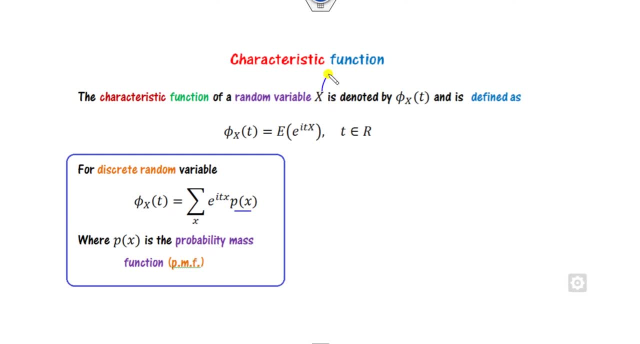 where px is the probability mass function of this random variable, x. On the other hand, if you have the continuous random variable, then instead of this summation, you have to write this integration. Now, our target is to write the characteristics function of this probability. 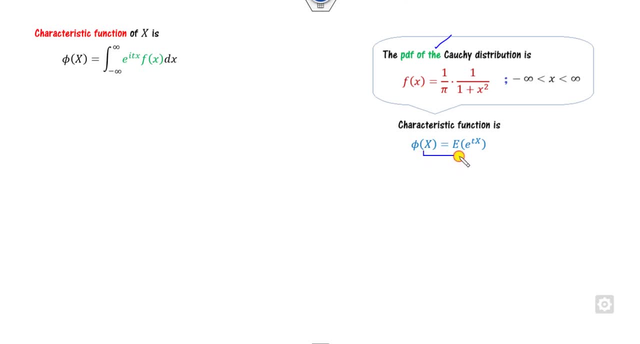 density function f of x. So as per the definition of the characteristics function, we can write like this: We can substitute the value of the f of x from here, 1 by pi is a constant which can be taken outside. Now the major thing arises is how you can solve this integration. because of this, 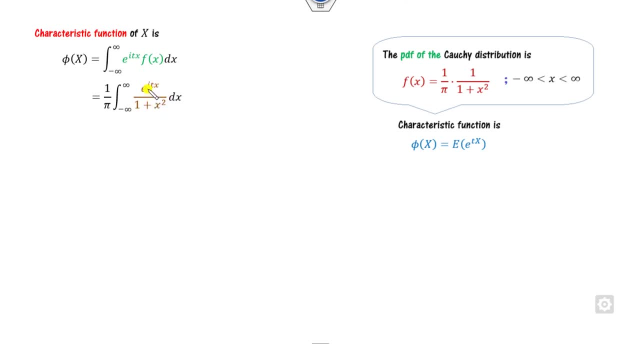 exponential and there are so many singularities are there because it's a complex part, So clearly says that how many singularities are there. it is my plus minus of iota. So it means you have to apply the complex analysis theory. The first method is you can use the residue theorem of the complex. 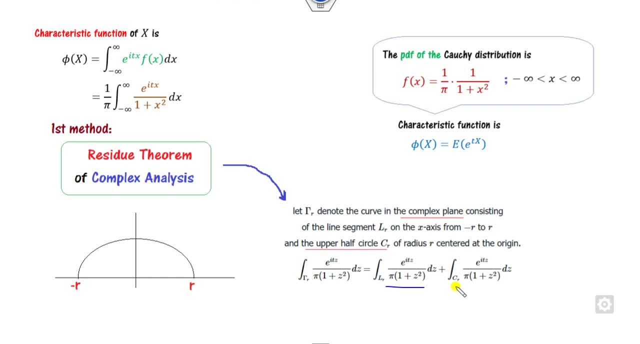 analysis like of this, which can be integrated like this, but once you are apply the residue theorem it you have the vast knowledge about the complex analysis. but those students who are unable to remember the complex analysis, in that case this integration or this theory will not be work for you. 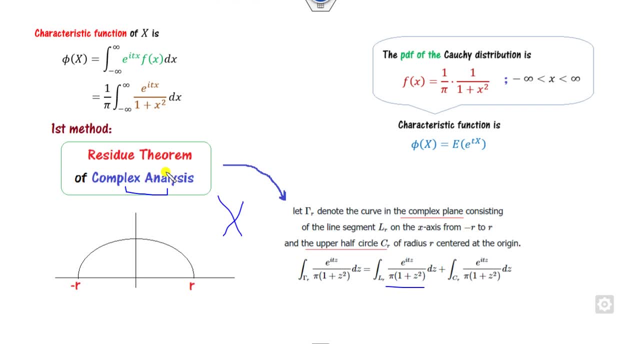 then we have to apply the second method, which is quite easier as compared to this first method, which is here. We can consider any of the function f of t as here. then we can apply the Fourier transformation, So we can compute the Fourier transform of this function f of t and then we can. 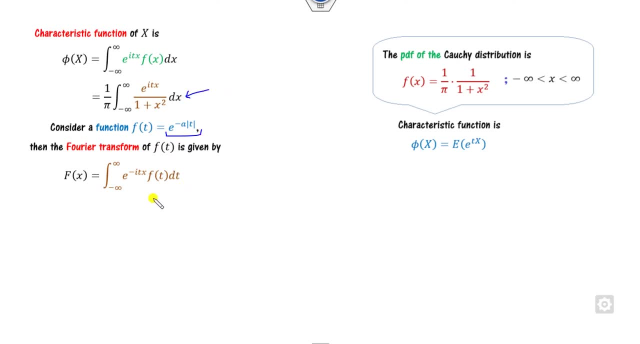 find the characteristics function from here, How we can see so I can substitute the value of the f of t. that is a Fourier transform here. now it is a mod of t, so we can break this integration into two parts, from minus infinity to 0 and 0 to infinity. when it's a minus infinity to 0, it's this mod of t is my negative, so it's a. 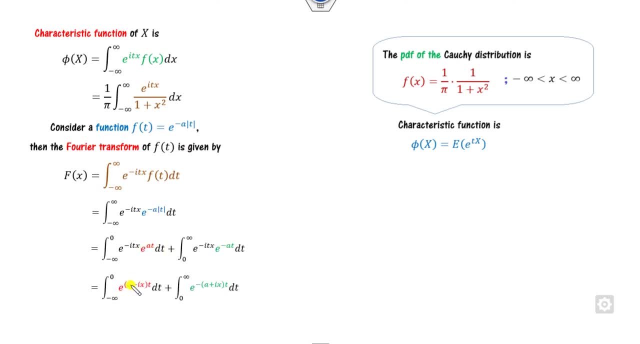 minus, minus plus, and so we can take the pair here. now how you can integrate them. so it's an exponential part you can easily integrate, which is here. when you substitute 0, the answer will be 1 over this. when you substitute minus infinity, it will be my 0. similarly, for this part, when you substitute 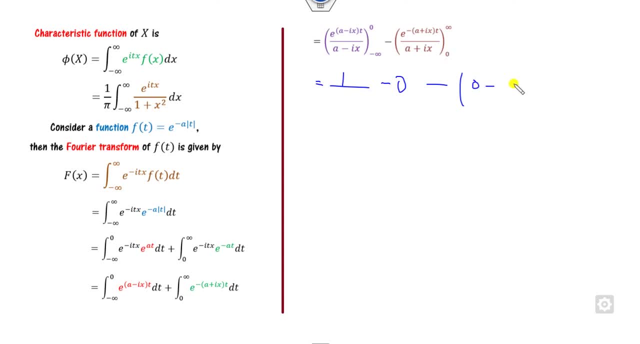 infinity, it will be 0 minus. when you substitute 0, it will be 1 over something. so you can see it's a minus minus, plus. and here now, if you take the LCM, you will get this part. so if you closely look about that, it is much similar to this part. now, here we have taken the Fourier transform. 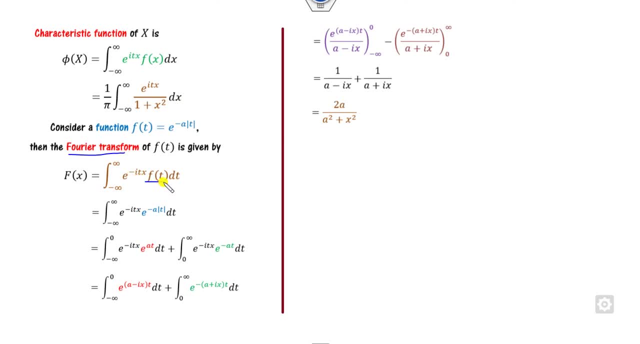 now you can find the function value. our target is to find the function so we can take the point delta zero and the multi want love t, which is 0, our stranger here- and the. those are digital Boxes, toinos, characters, so those are good for terms of this table. so在利息 gap as the dual. 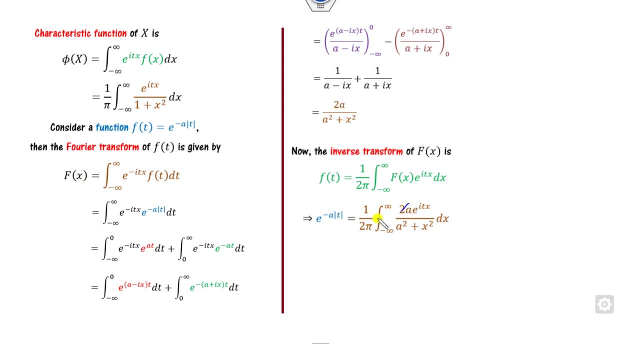 Oxyrhos on white sphere. these colleagues, now it's called at rights, natürlich latex. and if you compare this with under a negative好, this is the square root over likely conservation of f from right side to the guilt here which isしま clock, dash side is notыш. 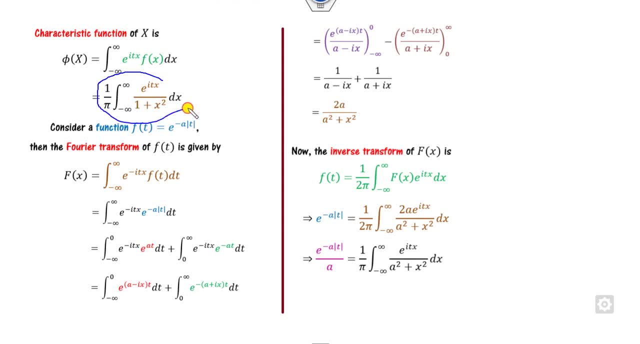 left hand side, so you can see this part is completely observed from here. so what is the difference between them is, if you simply take a is my 1, then you can say: this portion and this portion are similar. so if you take, a is equal to 1, so this portion is nothing but my here. 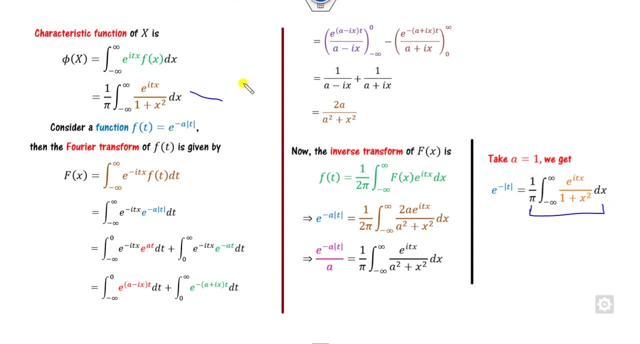 what is that? if you compare this equation number 1, if i write this is equation number 1 with here, this is nothing but my characteristic function of this cauchy distribution. so this is the simplest way you can solve this cauchy distribution characteristic function instead of any of the 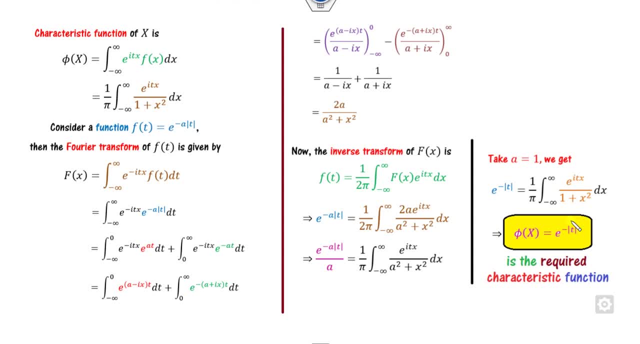 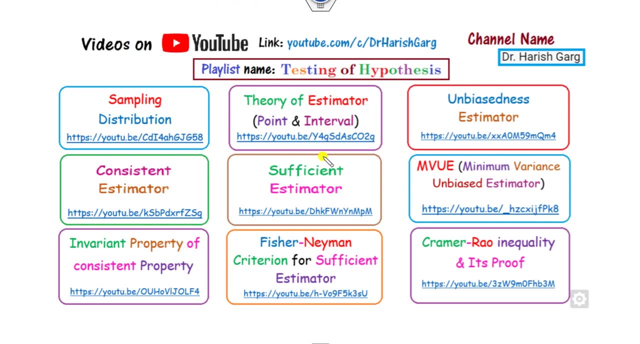 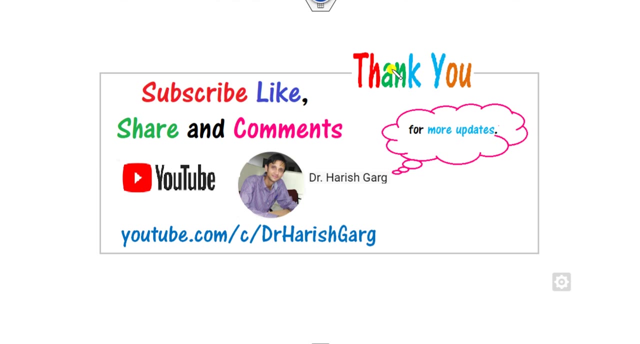 complex analysis: residue theorem. i hope you can simply learn this simple trick from this video. if you find some another video like testing of the hypothesis consistent estimator grammerau, newman, principal, mr, you can simply follow my channel name, dr harishkar, and so on. i hope you can like, share and comment.